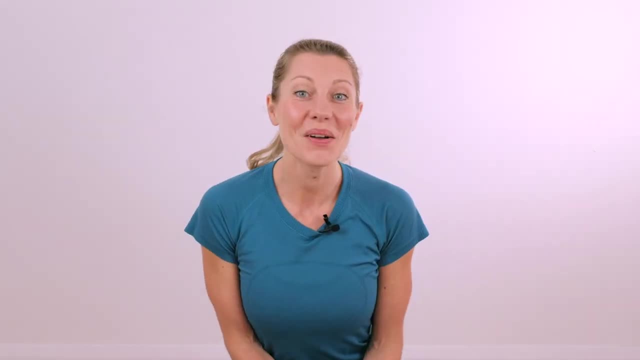 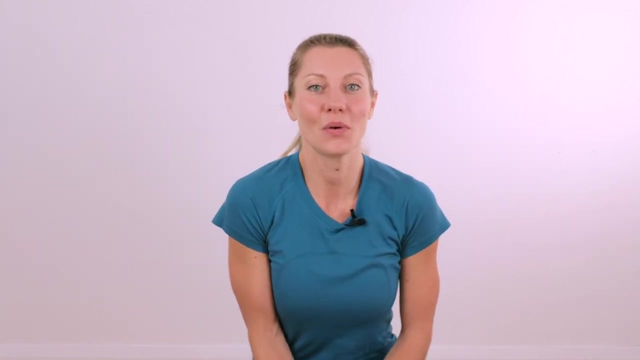 Hello everyone. it's Helen from Class Yoga. So today we're going to do a lovely class that's all about relaxing and helping us to feel good and nice and calm. Great, if you're feeling a little bit tired, a little bit grumpy, I'm sure it'll help you feel much better. 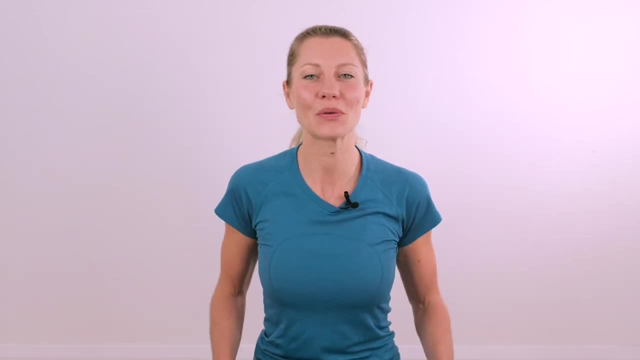 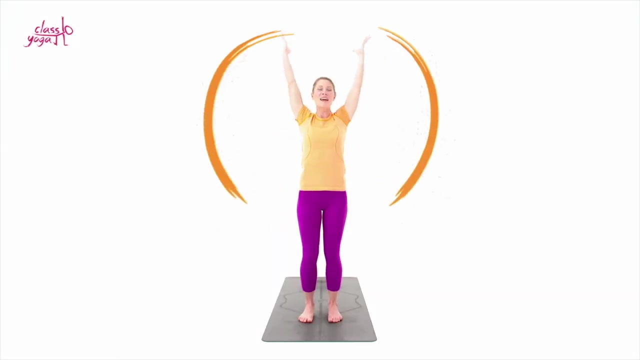 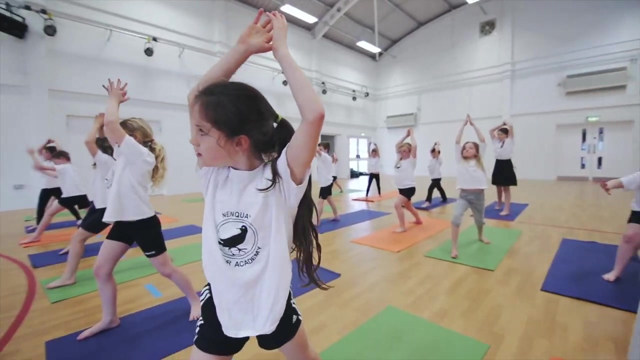 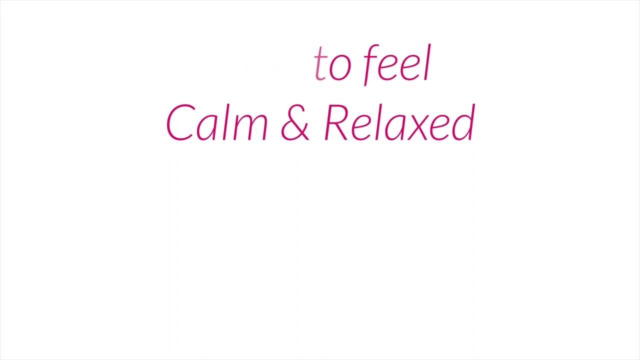 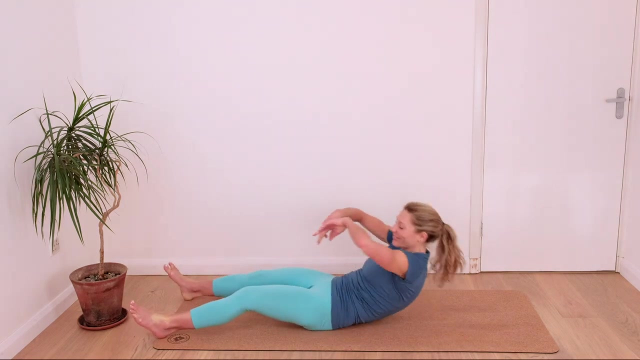 So grab yourself a mat or find a nice space to move and we'll get started. Okay, everyone, let's start lying down on our back. You might like to take a long stretch out to begin. Ah, and bring your hands onto your tummy, Bring your fingertips together. 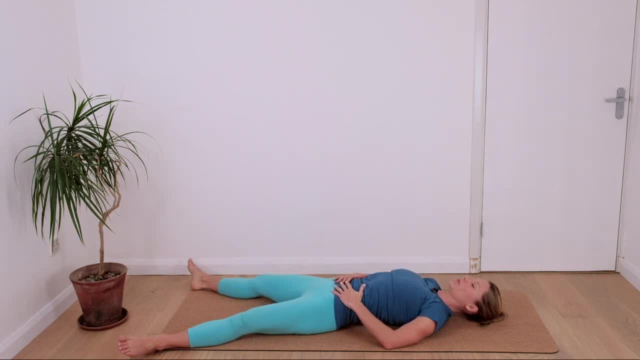 And as you breathe in, feel your belly up and then let it go down A little bit, like a balloon breathing in, fill it with air, Ah, and then feel it go down. So your fingertips might touch here as you breathe in. 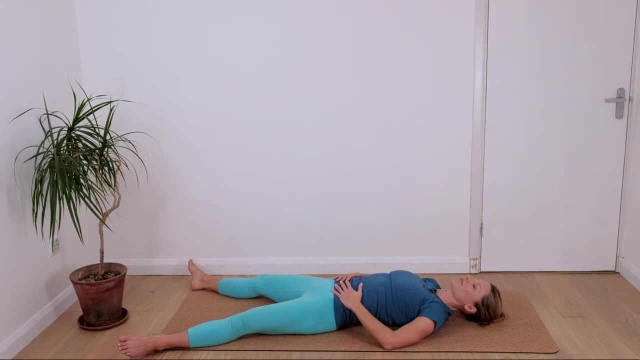 And as you breathe in, they might move apart. Let's just take a few more breaths here. Notice that, See if we can begin to feel a little bit calmer. Ah, and forget about the rest of our day just for a few minutes. 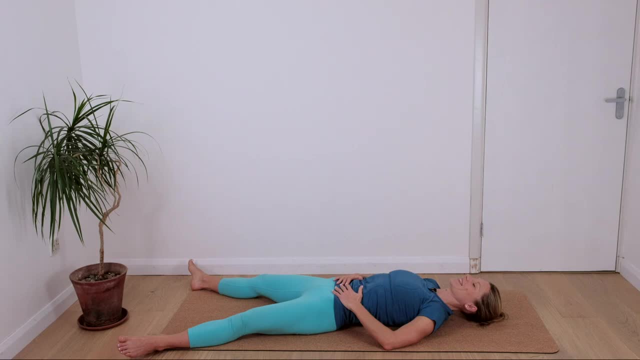 Good, everyone. Okay, bring your knees in towards you and take your head up and make yourself as small as you can, And then as long as you can- Again, as small as you can, And as long as you can. Once more. okay, from here let's go into a little bit of a banana shape, take your feet to. 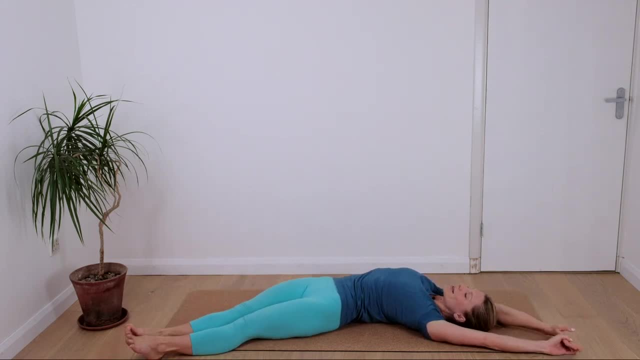 one side, your arms to one side, but let's keep looking up and keep on back on the floor. two or three big breaths along this side. it gets getting longer. great. back to the middle, then over to the other side, over with your legs, over with your arms, doesn't 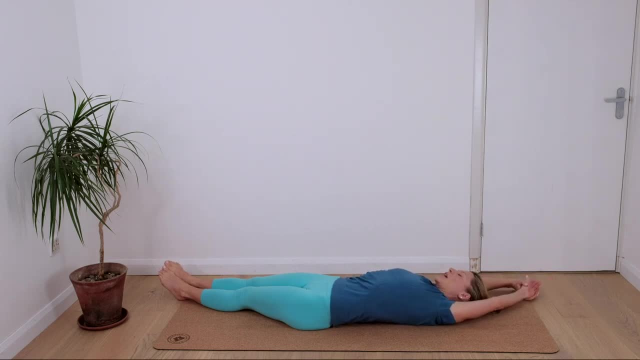 need to be very far, somewhere that feels nice. maybe you get a little bit of a stretch down this one side. that's getting longer. Good, let's come back to the middle. bring your arms down, let's roll over and push yourself up. Come and take a seat, cross your legs, open your arms out wide to the side and then give. 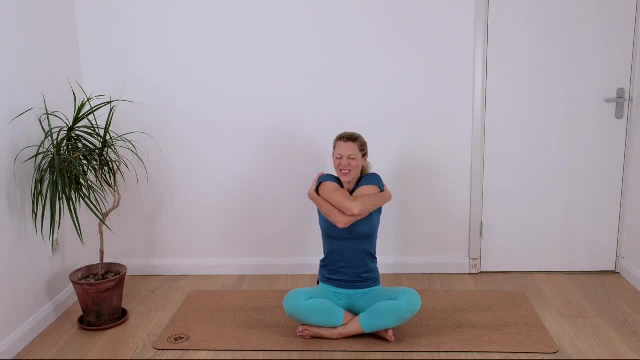 yourself a hug, really big hug. see how you're feeling and either stay here with your arms or wrap your arms around. Then we can fold forwards a little bit, you can drop your head, you can close your eyes- Good- And then roll back up, open your arms, uncross your legs and switch them the other way round. 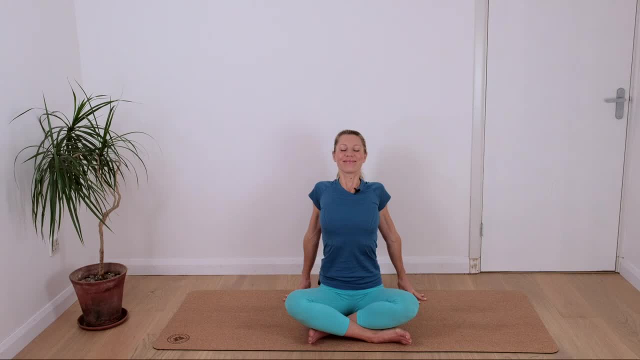 lift your chest a little bit, Open your arms again and we want to try and cross them over the other way round. Nice, big hug, a big squeeze, Just for you, And then stay there or wrap your arms around again. We could fold forwards, drop our head a little bit and then let's come back up, open your 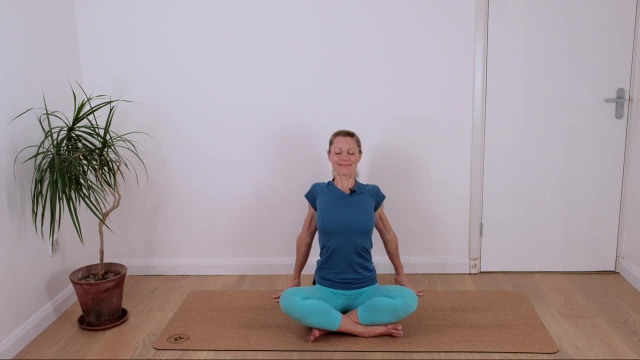 arms. Lift your chest. Okay, so we're going to stay. see, let's come onto our back, Feet to the floor, hands to the floor, and we'll take a little bridge lift. Let's lift our hips and tummy up. 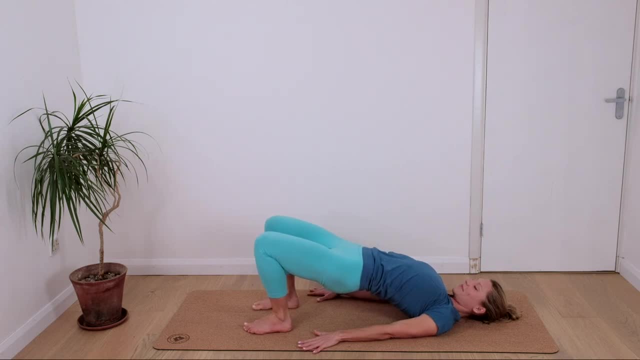 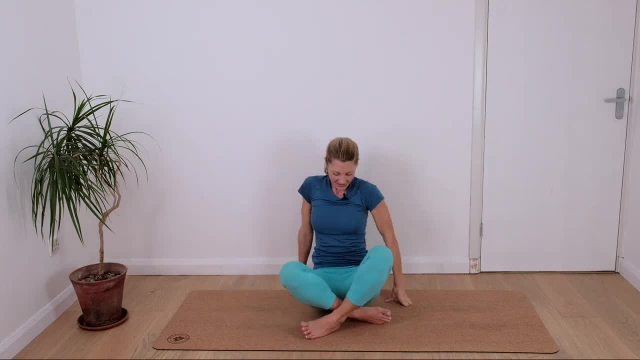 Come back to your seat seat. Okay, let's use our fingertip to close our right nostril and breathe in our left one. Close that one and breathe out the other one. So we're drawing a mountain. Breathe in and breathe out the other side. Imagine you're going up the mountain and down the 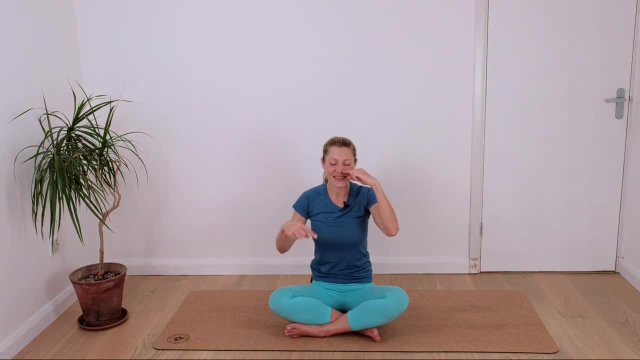 other side, Up and down. Let's try it once more: Up and down. Let's see if we can come down the left side And then relax, Close your eyes, Notice how you feel just now And take a long reach all. 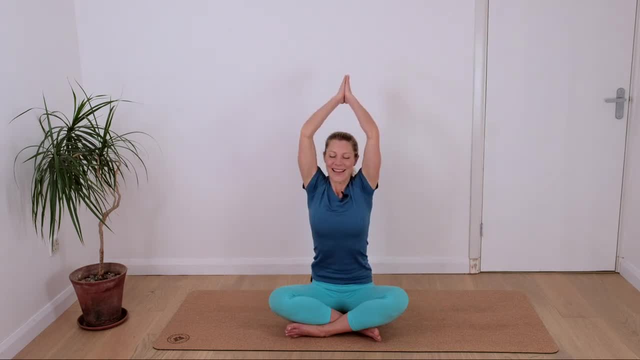 the way up And back down. Good, All right, well done. So how do you feel now? Let me know in the comments below. Let me know if you like this video by clicking the like button And subscribe to Class Yoga on the red button just underneath And I look. 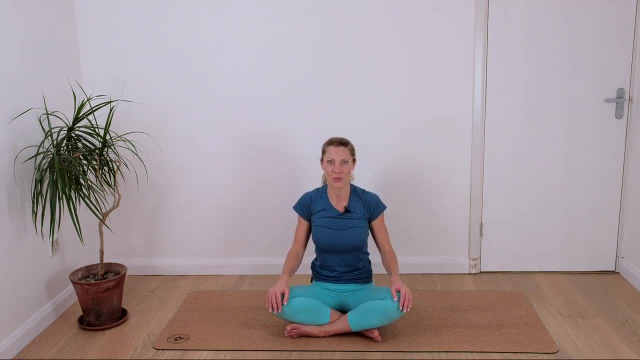 forward to sharing more real yoga for kids with you.